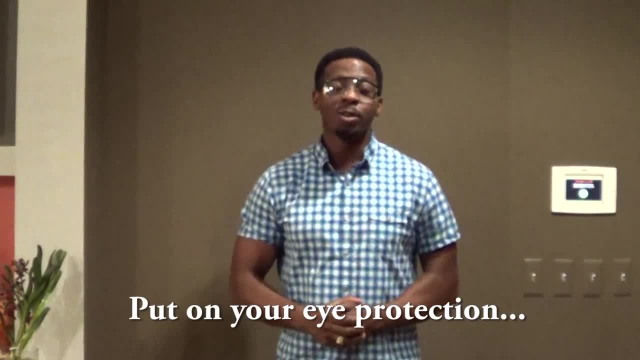 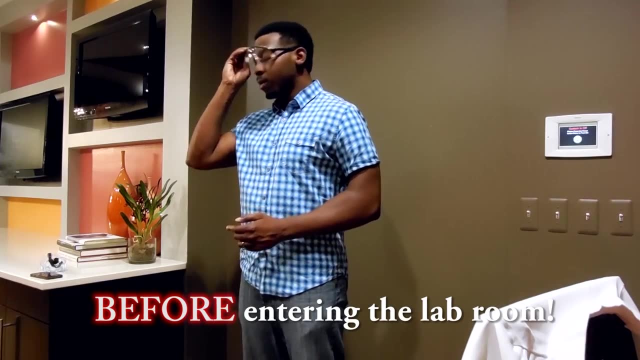 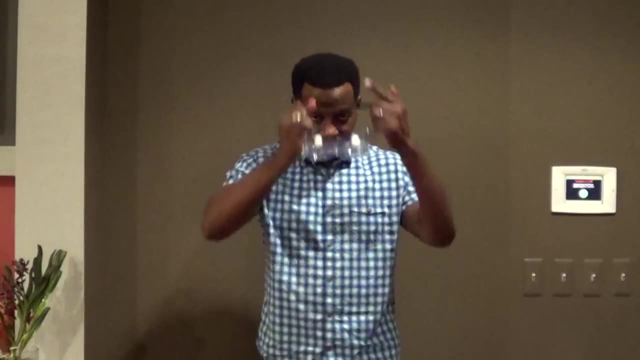 me against projectiles that may fly in my eyes so that I don't lose my eyesight. However, if you're using chemicals, you want something even more powerful than safety glasses. You want these. These are splash goggles. Splash goggles provide you with the same protection as safety glasses will, but in 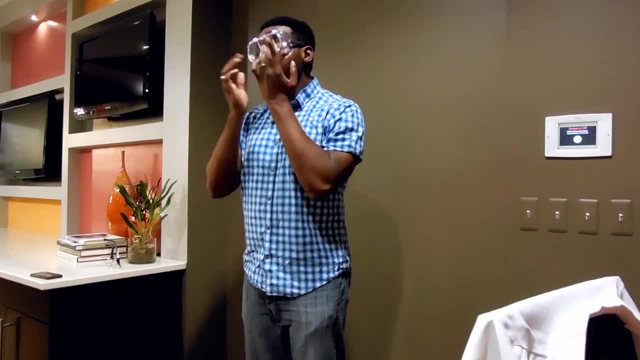 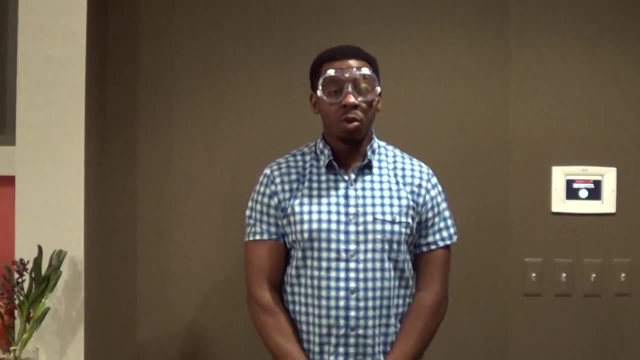 addition, splash goggles are covered all the way around the rim against your face, so that if a chemical splashes, it won't get onto your face or onto your eyes, where the goggles are present, And so it's very important for you to know the difference With the wet chemicals. 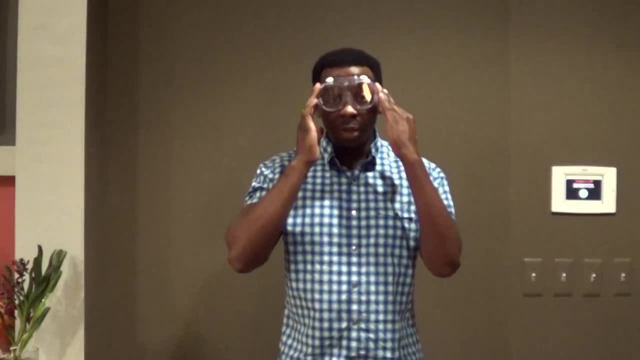 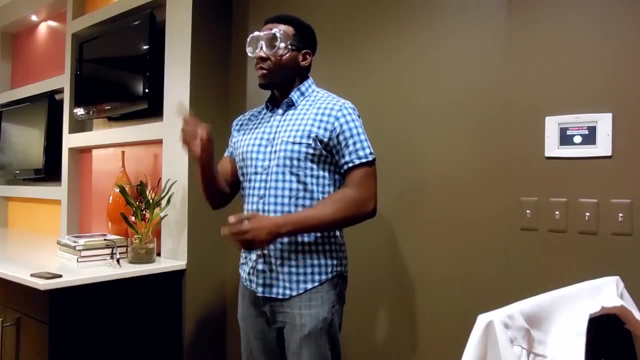 that can splash. I definitely want to have on my safety splash goggles. If I'm not using wet chemicals, then the safety glasses may be okay. The next level of safety that I have to employ when I go to the lab is this handy lab coat. 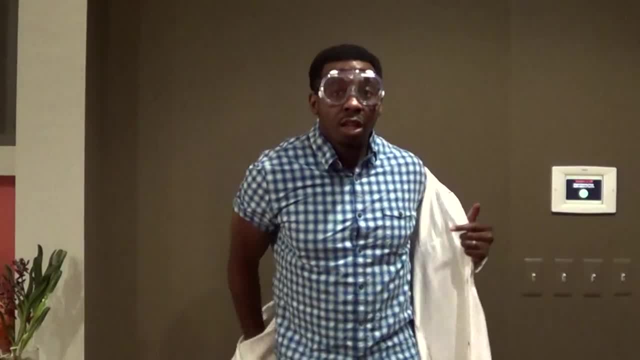 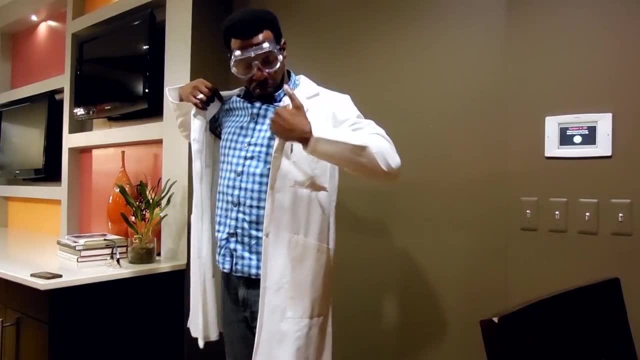 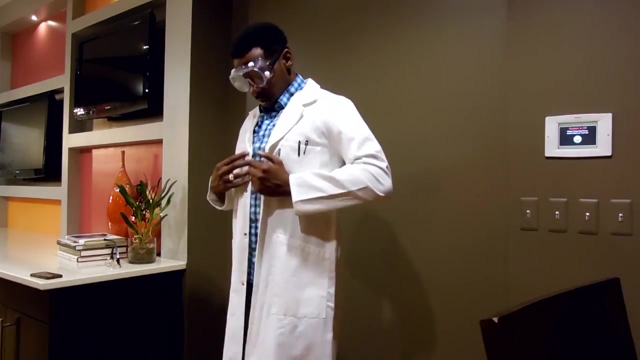 Now, the lab coat will protect me- my clothing- from getting chemicals on it, especially if something splashes on me. So it's important for me to wear this, because I don't want to take the chemicals from my lab home with me. I don't want them to get on my clothes. So 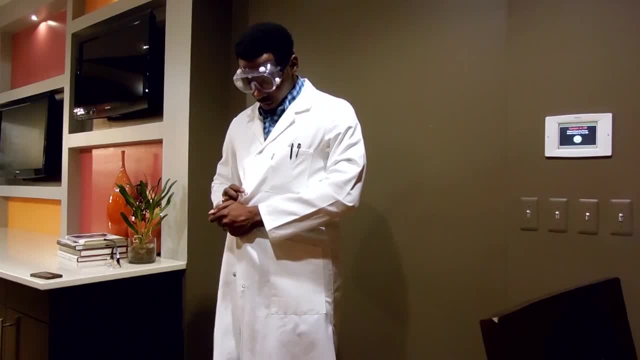 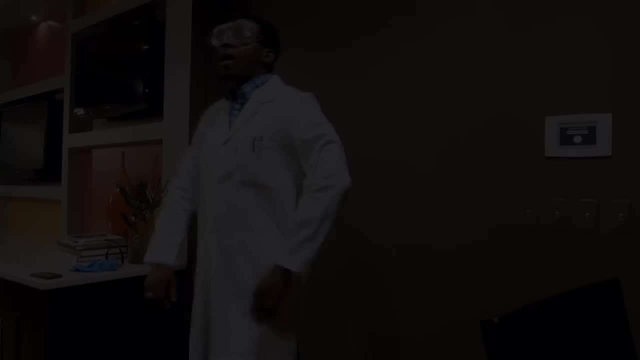 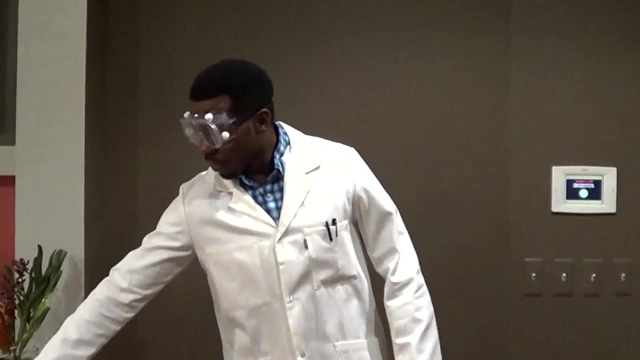 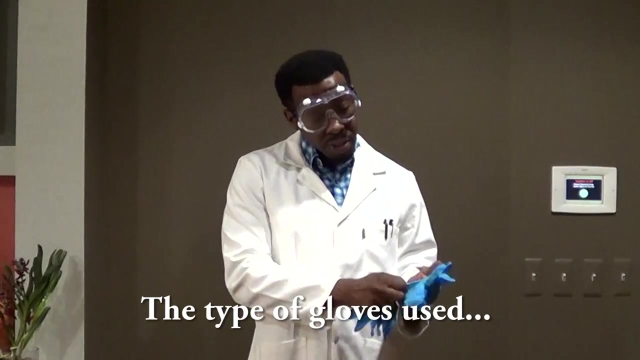 as much as is possible. I want to be completely covered up with a lab coat, in addition to my splash goggles or my safety glasses. Finally, if I'm working with chemicals, I definitely need to cover up my hands. That's why we have gloves Now. the safety gloves are designed to protect my hands from getting 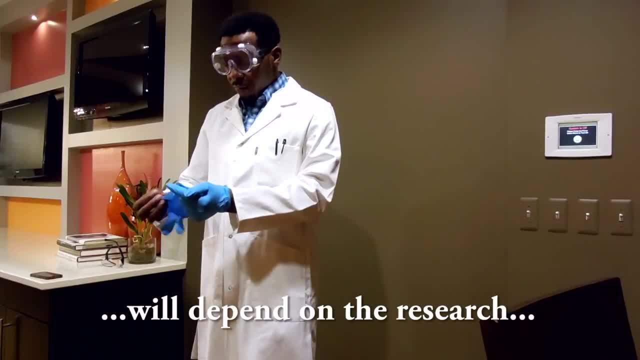 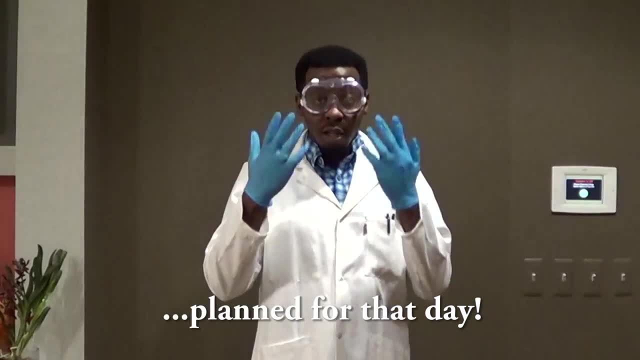 chemicals on them, And this way, my skills aren't just going to go to waste. Now, the My skin won't be harmed, my fingers won't be harmed and I won't be rubbing my eyes with something later on. that's on my hand. 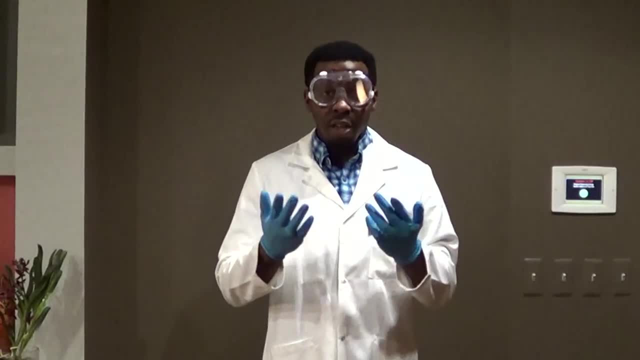 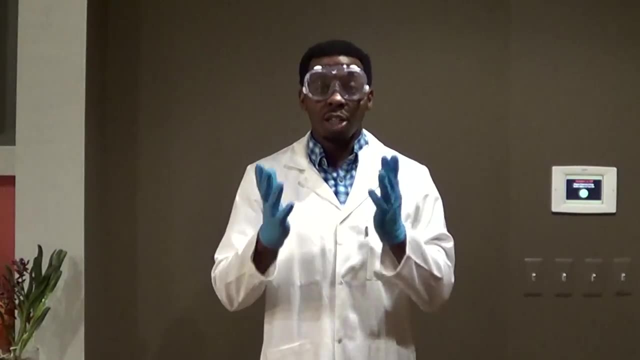 Now make sure, when you're wearing your safety glasses, your safety gloves and your lab coat, that you're still careful how you pick things up and how you handle them. You still, because you have the gloves on, you still don't want to rub your face at all.